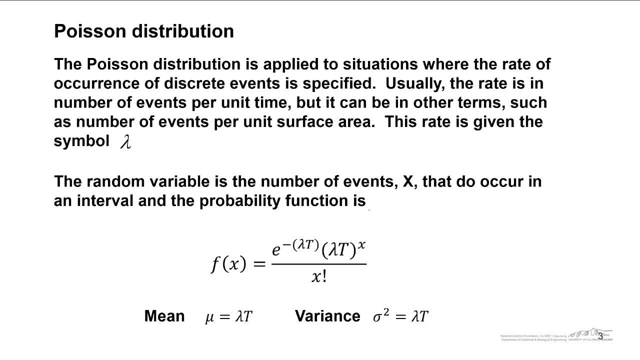 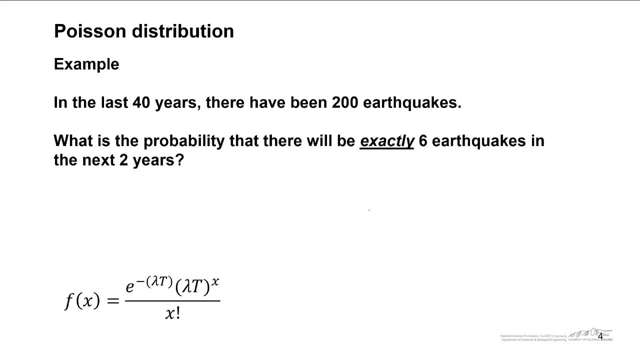 the probability of getting X number of events in a continuous interval. The mean is lambda times T. T is the period of interest. You can plug that in here and you can estimate the probabilities of a certain number of events occurring in an interval Using the Poisson. 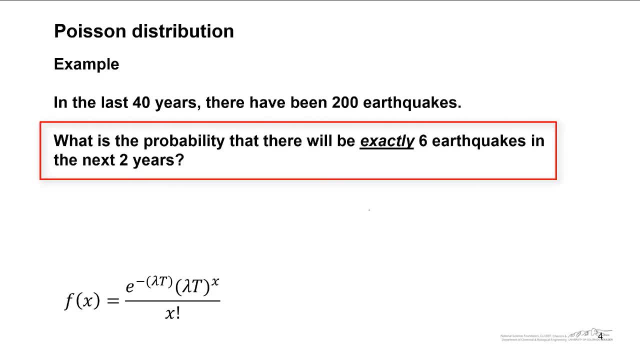 distribution. we answered questions like: what is the probability that there will be exactly 6 events or earthquakes in the next 2 years? And what we did was we calculated a background average rate of occurrence: 200 earthquakes or events per 40 years and that's 5 per year If we 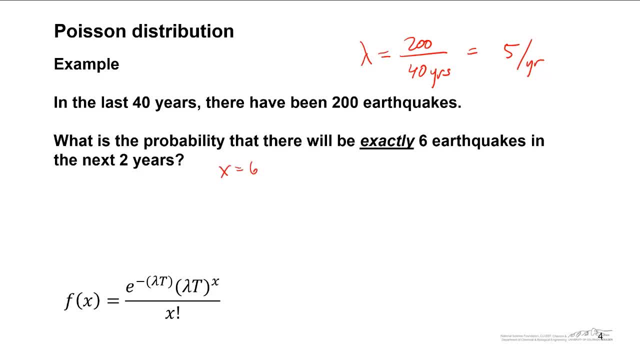 want to answer this question. X would equal 6, exactly 6 events or earthquakes. Our time interval would be 2 years. Lambda t, which is also known as the mean, is equal to, in this case, 5 times 2,. 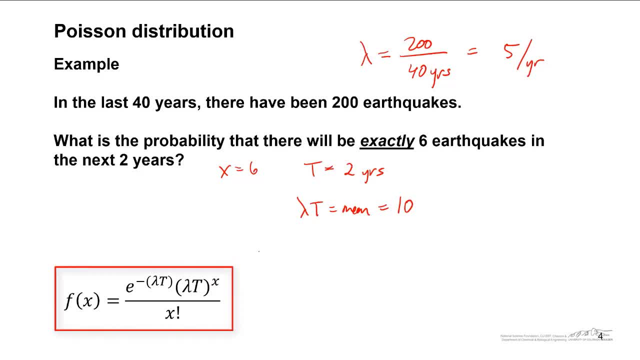 and that would be 10.. into this function, with x equals 6 and when you do this you would get about 6.3 percent. there's a 6.3 percent chance that in the next two years there's going to be exactly six earthquakes now. 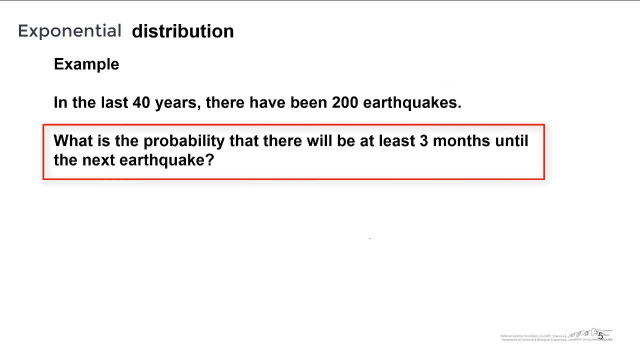 what we're going to do is we're going to ask questions like: what's the probability that there will be at least three months until the next earthquake? this is known as the exponential distribution, and x represents a continuous interval. in the Poisson distribution, x represented a discrete number of events, but in the exponential distribution, x is going to represent a continuous. 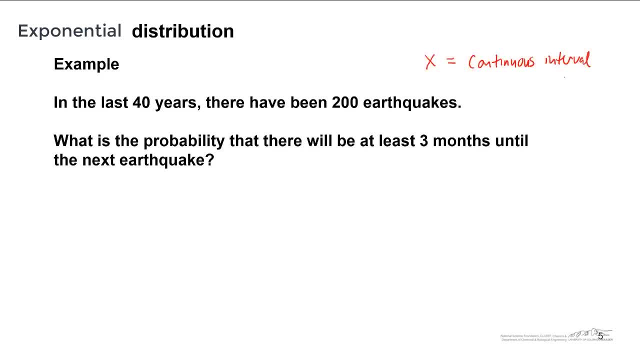 interval. so we're kind of flipping the Poisson distribution on its head and we're saying now, instead of what's the probability of getting a number of events in an interval, we're asking what's the probability of an interval between events. in other words, if we were to look at 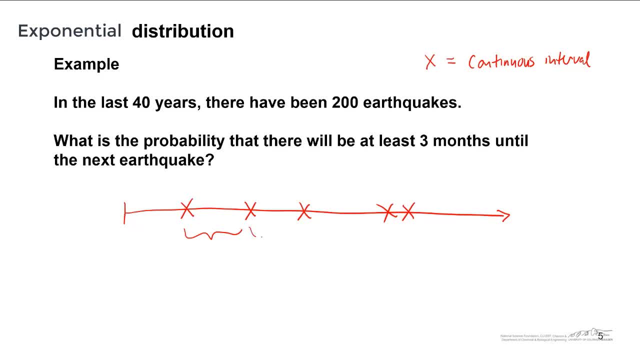 earthquakes, the exponential distribution would show up as a continuous interval. also, the knowing Evolving results result in a continuous interval and to do that we should be studying the Mib and his. The exponential distribution tells us probabilities related to the lengths in time, in this case, if this is earthquakes between events. 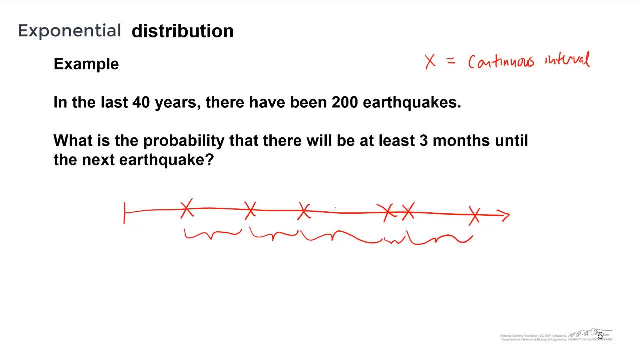 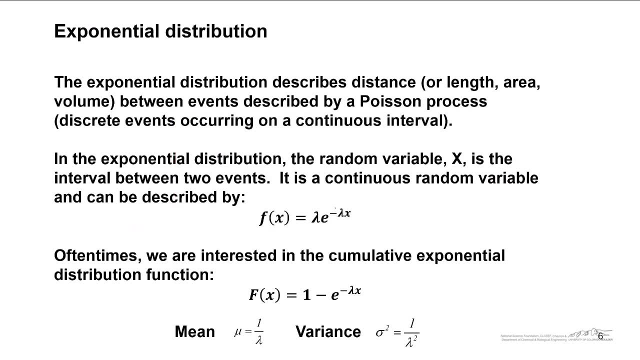 And importantly, it's always the interval between subsequent events. So the exponential distribution describes distance or length, area, volume or time between events described by a Poisson process, discrete events occurring on a continuous interval. The random variable x in the exponential distribution is the interval between two events. 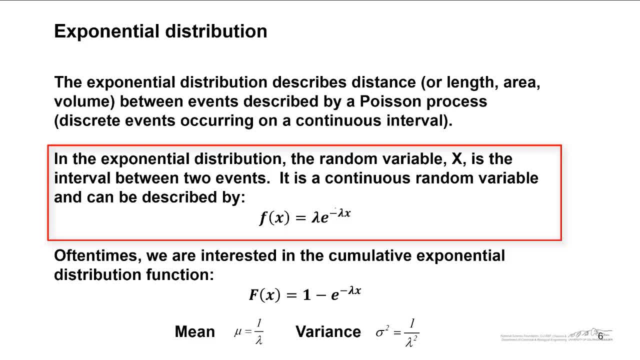 It is a continuous, random variable and can be described by this function. So this is just the little f, the non-cumulative. Oftentimes we are interested in the cumulative exponential distribution. So if you integrated this, if you integrated little f, you would get capital F down here. 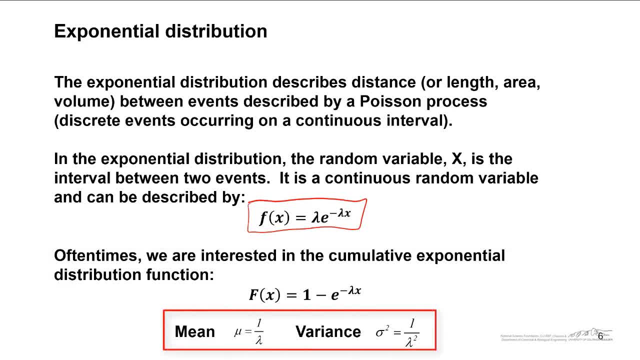 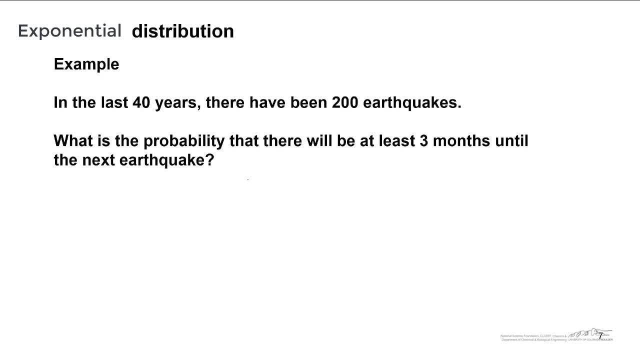 1 minus e to the negative 1.. So this is the cumulative lambda x. The mean of the exponential distribution is 1 over lambda and the variance is 1 over lambda squared. It's a lot easier for you guys to learn if I go through an example. 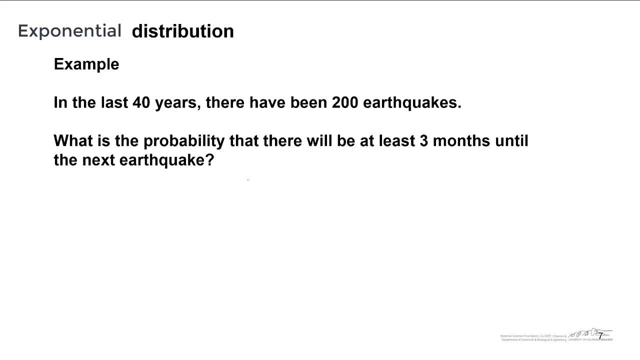 200 earthquakes in 40 years. What's the probability? that there will be at least 3 months until the next earthquake. x, then, is going to be 3, and it's not exactly 3,, it's at least, which means that we're going to be looking for the probability that x is greater than or equal to 3.. 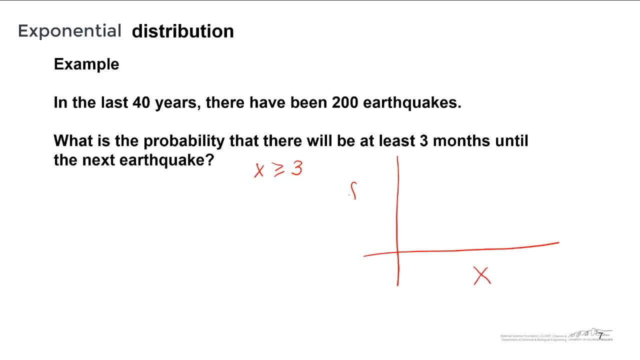 In other words, if we were to plot x, which is time, and our probability density function for the exponential distribution, the exponential distribution looks something like this: What we're interested in is 3 months. What's the probability that the next event will occur at least 3 months from now? 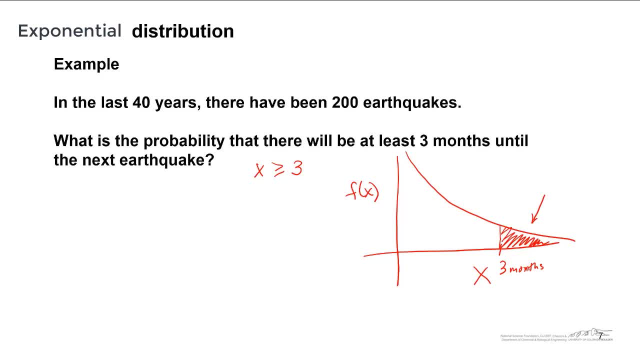 And so that's represented here by that shaded region. It could occur right at 3.1 months, but it could also occur 10 months or 100 months from now. So if we sum the area underneath that curve greater than 3,. 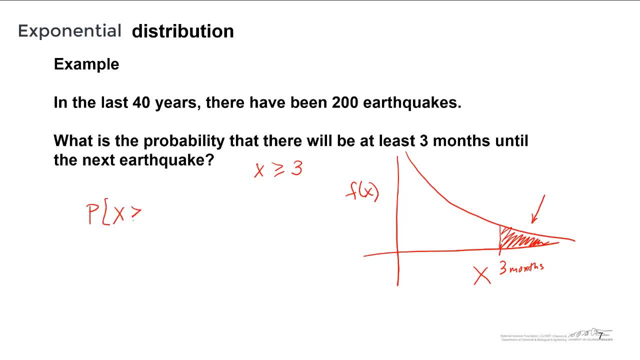 so what we're trying to find is the probability that x is greater than or equal to 3.. In terms of cumulative probabilities, how would we write the probability that x is greater than or equal to 3? This is the same as taking 1 minus the cumulative up to 3.. 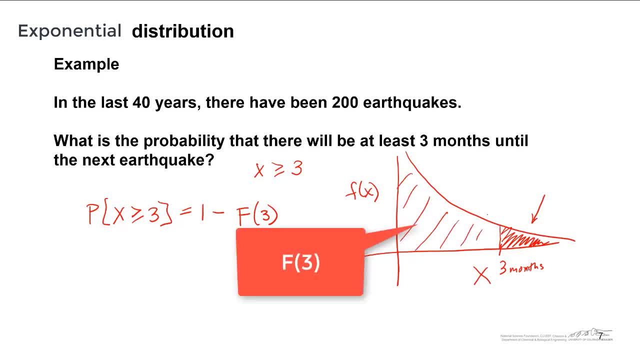 F of 3 represents this region here on the left. If we subtract that from 1, because the area underneath a probability density function is always going to be 1, then this will tell us what we're looking for. F of x is equal to 1 minus e to the negative lambda x. 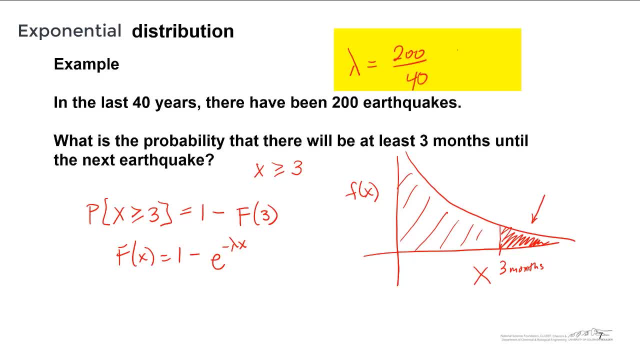 Lambda is going to be 200 divided by 40, which is 5 per year. We want to make sure- because x down here is in months, we want to make sure that we convert this to months So we can multiply 1 year per 12 months. 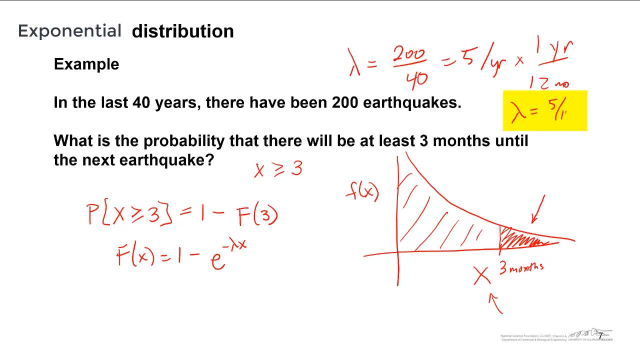 and really lambda- is equal to 5 over 12.. When we plug this into the cumulative function down here, when I substitute capital F of 3 into here and I subtract from 1, these ones will actually cancel and what we end up with is the probability that x is greater than or equal to 3. 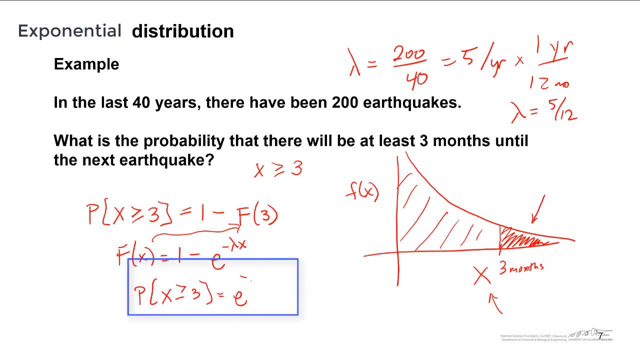 is just e to the negative lambda. x Lambda is 5 twelfths, Our x value is 3.. And when we do that, we get the probability that the next earthquake is going to be greater than 3 months. So it's going to be about 3 months from now, to be about .287.. 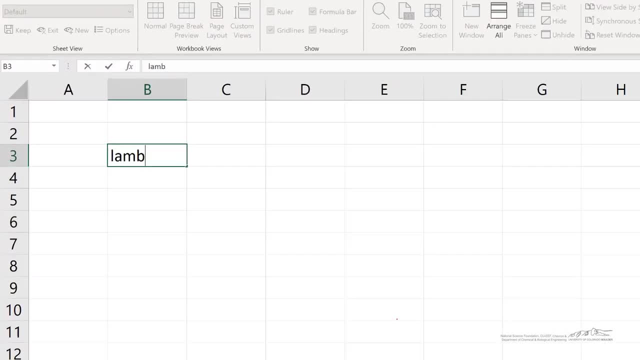 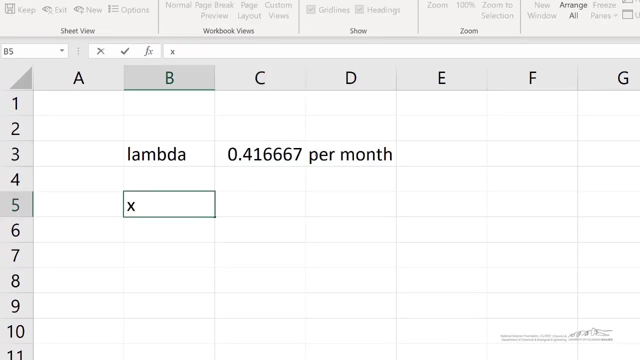 Let me show you how we can do this in Excel. What I'm going to do first is I'm just going to put in a cell here for lambda, and that equals 5 divided by 12, and that's per month. Our x value is equal to 3 months. 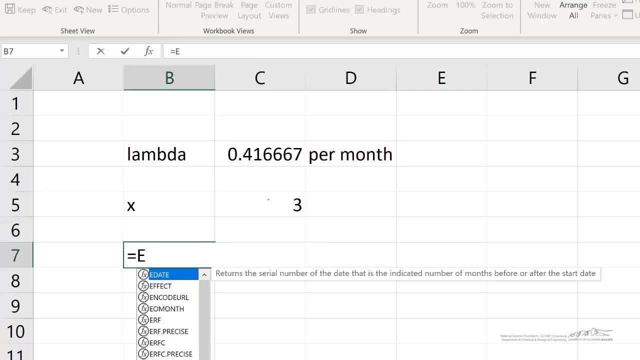 and we're trying to calculate greater than 3 months. So I can use the exponedist function in Excel. The x value of interest is 3.. Lambda is up here. I've calculated 5 over 12, and I want to do cumulative. 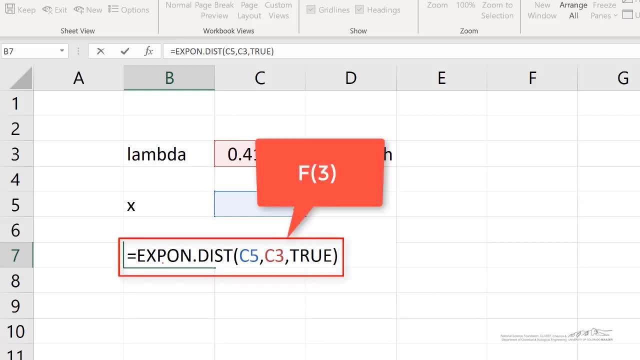 So this would give me capital F of 3 up to 3, but in order to get greater than 3, I have to subtract that from 1, and we get the same result that I did using a calculator. Let's go through one more quick example. 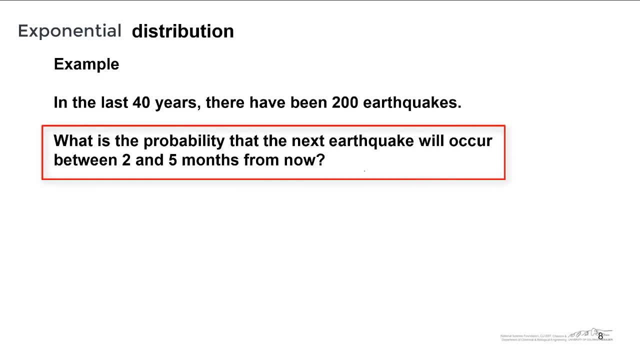 Same scenario: What's the probability that the next earthquake will occur between 2 and 5 months from now? Again, we have x in months. We have little f of x here. The exponential distribution looks something like this and we're being asked: what's the probability that, starting now,